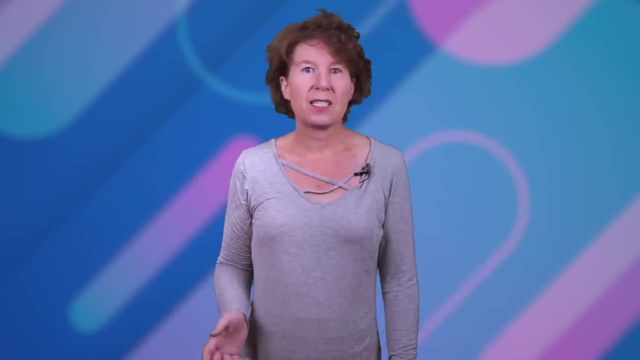 particles are the momentum of an object. Let's just pretend the massless particles are the momentum of an object. Let's just pretend the massless particles are the momentum of an object. Quantum mechanics says that you can't measure both the position and momentum. precisely This. 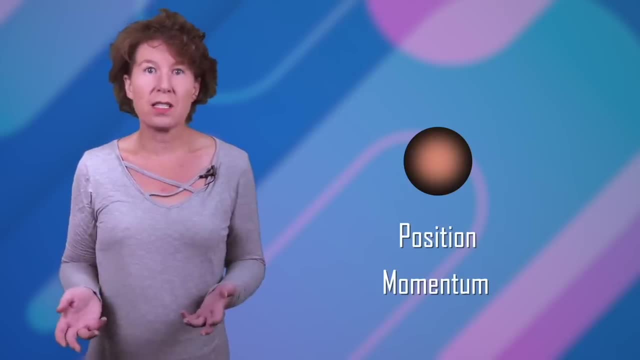 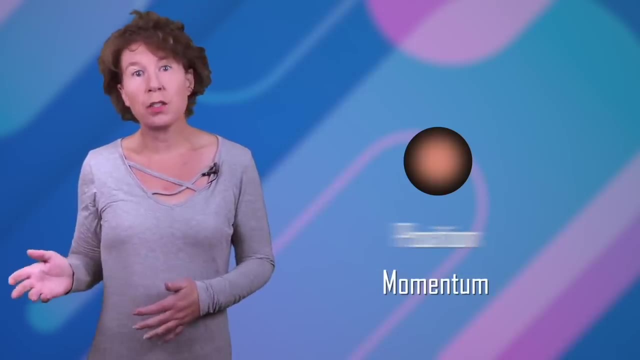 means: if you know precisely where a particle is, you don't know which direction it's going. And the other way around: if you know which direction it's going, you don't know where it is. The position of a particle is usually denoted with x and the momentum with p. 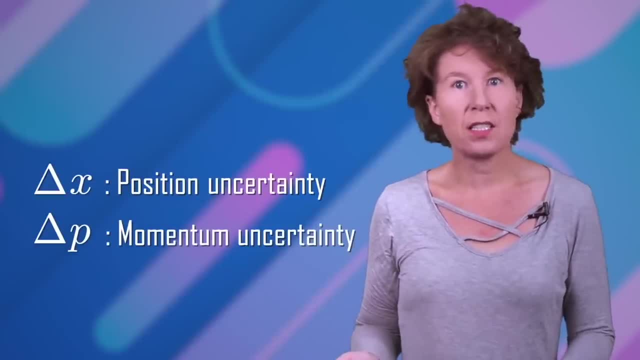 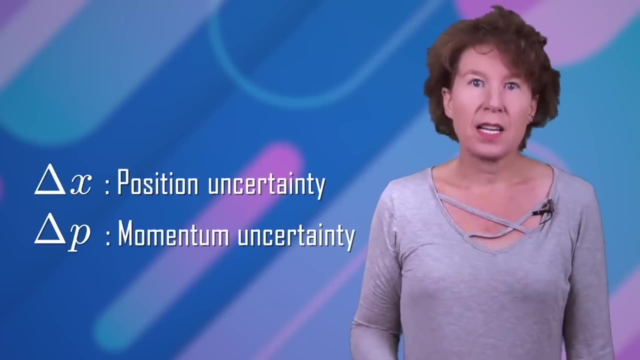 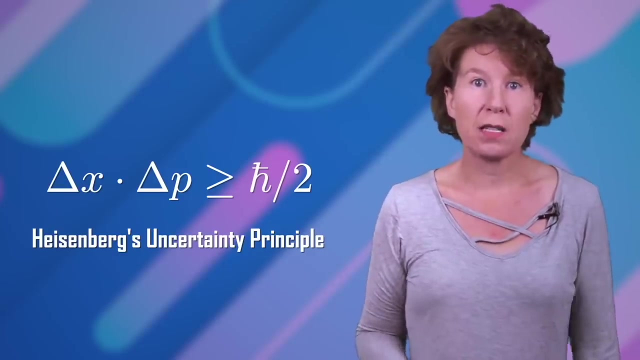 The uncertainty in each is marked with a large delta. Delta x is the position uncertainty and delta p is the momentum uncertainty. Heisenberg's uncertainty principle then says that the product of those two is always larger than a constant h bar divided by two. This means, if one of those uncertainties gets very small, then the other one must be very large, otherwise the inequality would be violated. This is where the joke about Heisenberg comes from, where he gets stopped by the police who tell him how fast he was driving, and Heisenberg says: great, now I'm lost. 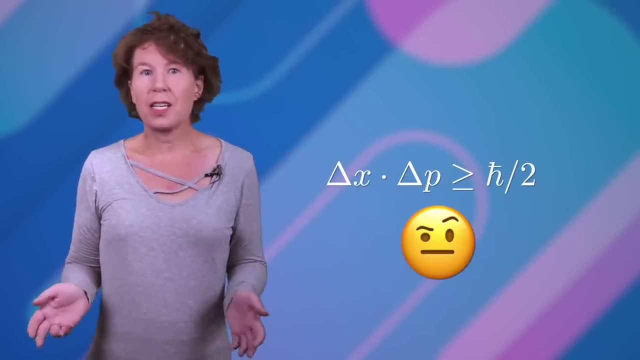 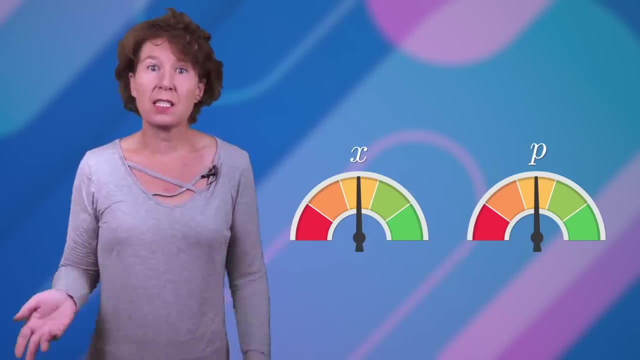 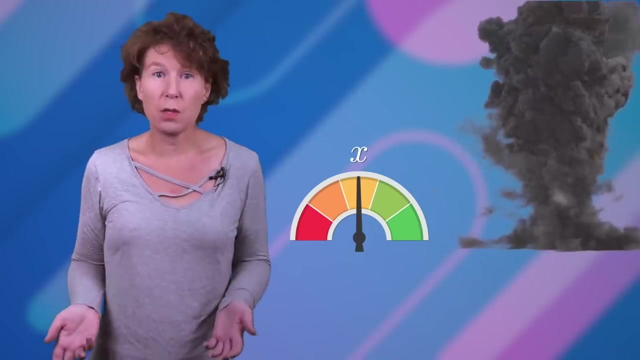 But what does it mean? that you can't measure the position and momentum with certainty at the same time? Does it mean that if you come with two detectors, a lightning strike will explode one of them? Well no, The uncertainty principle doesn't say that you can't measure both of those quantities. 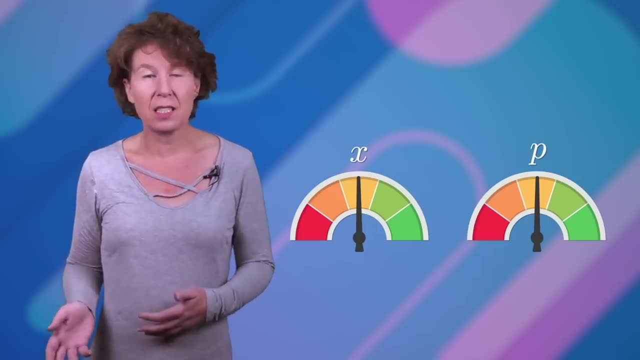 It shows that you can't measure both precisely. If you've pinned down the one, then the other will have a large spread. This means if you repeat the experiment, the result will be all over the place. It's the statistical uncertainty of this series. 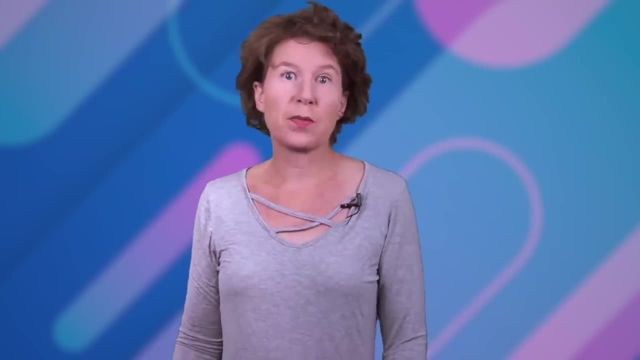 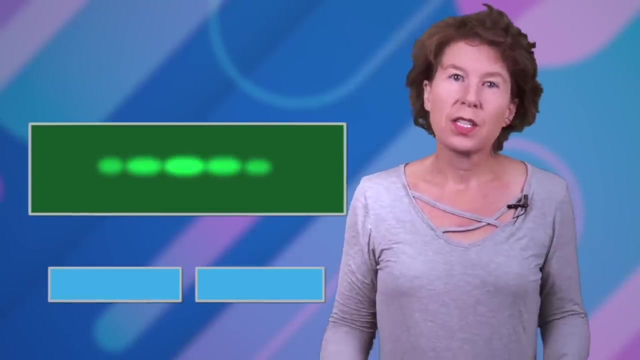 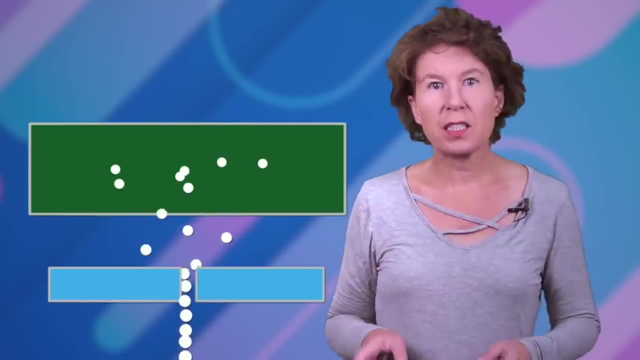 of measurements that becomes large. A good example of this is letting quantum particles go through a narrow opening. The quantum particles act like waves, So this will create an interference pattern on the screen. This pattern is built up of single particles. The particles don't all collect in one pattern. The particles don't all collect in one pattern. 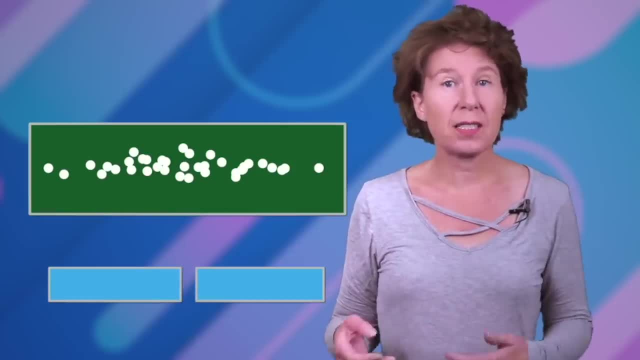 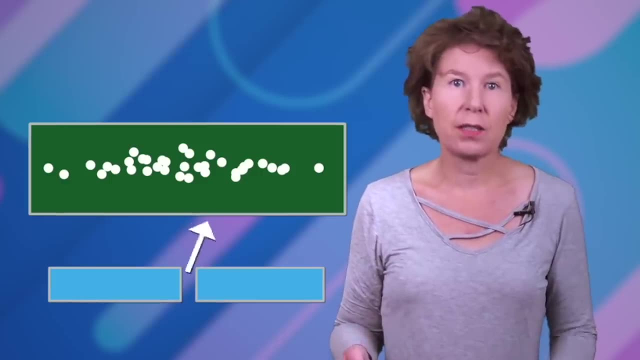 And that's because you know the particles went through the slit, so you know something about their position. Then you can't tell which direction they are going, But of course, once a single particle hits the screen you know which direction it went. What the uncertainty. 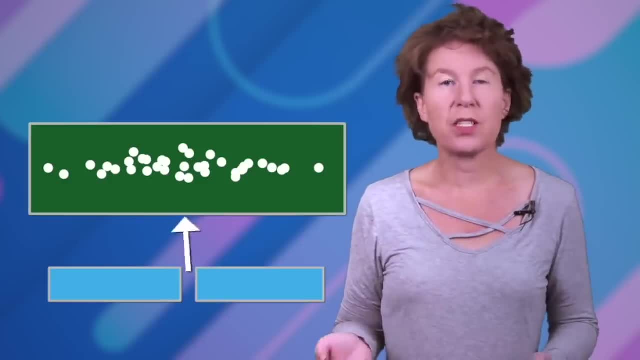 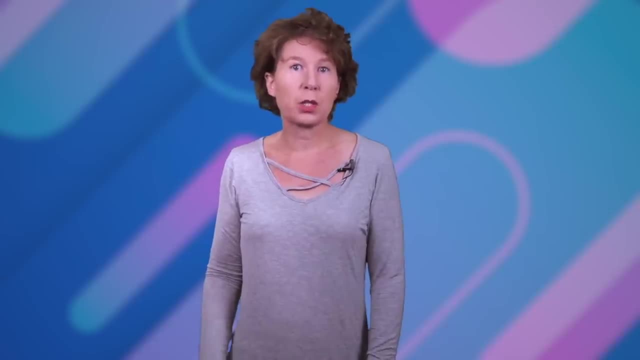 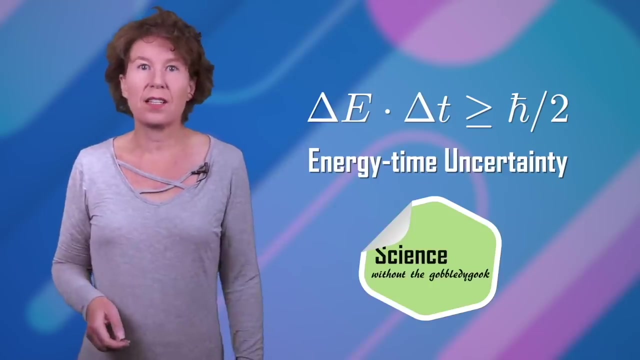 principle means is therefore that if you repeat this for many particles, then the outcome has a broad distribution. Another example is the relation between the uncertainty in energy and power. Consider: you have a fluorescent sticker, the kind of stuff that glows in the dark. 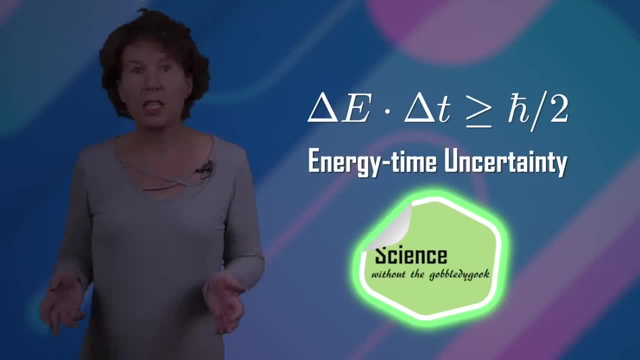 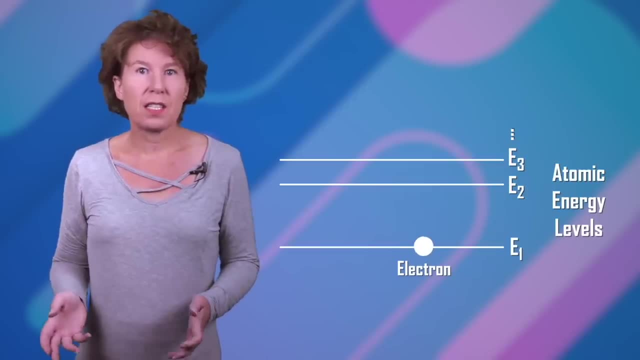 You put it into light and then for a few hours afterwards it'll emit light of a particular color. usually it's some shade of green. The way this works is that the light which falls on the sticker kicks off an electron from its normal energy level into a higher. 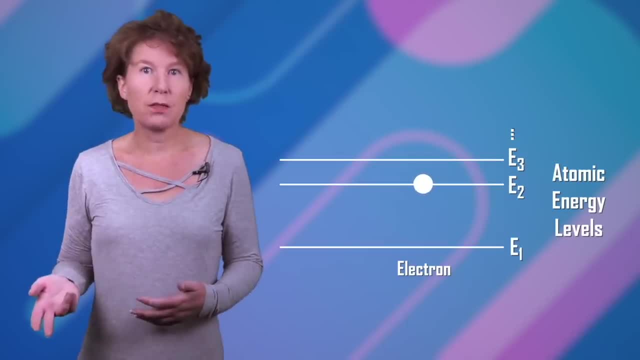 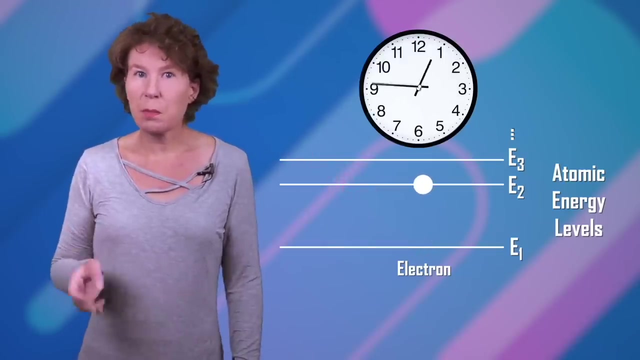 level. In most materials, the higher electron levels are extremely unstable. The electron falls back down immediately And in that process the photon is emitted again. In fluorescent materials, however, the electrons can stay there for a few hours. It's called a metastable state, And only 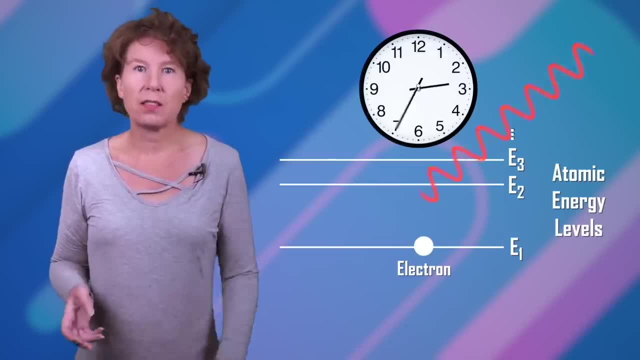 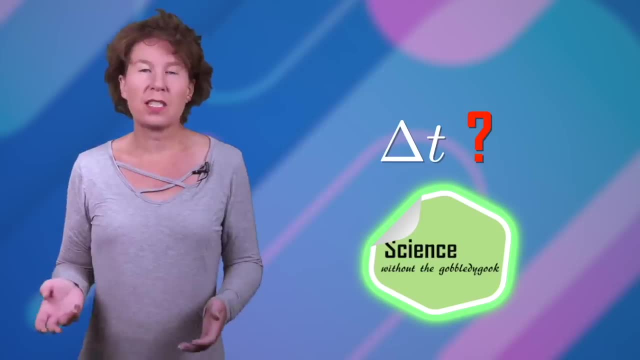 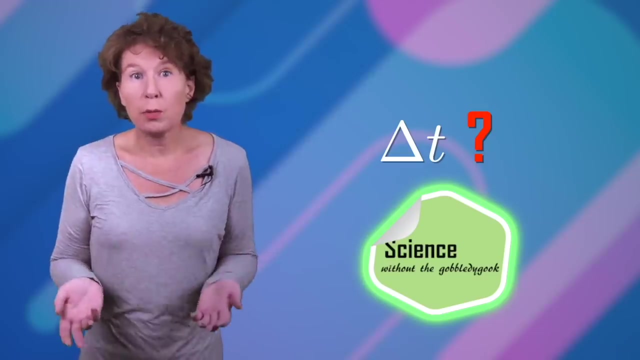 when the electron falls down, will the light be emitted again. As a consequence, the sticker glows for some hours. But just exactly how long do the electrons stay in that higher energy level? Ah well, you can't say exactly, You can only talk about the probability. 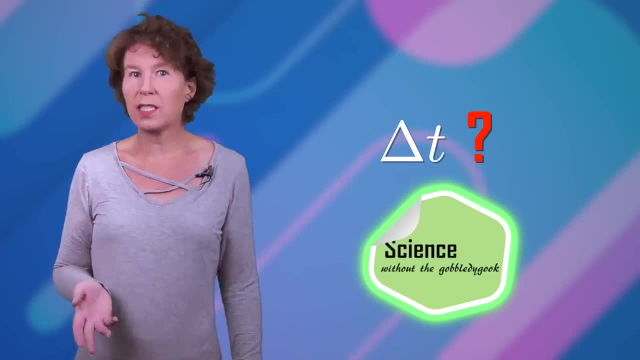 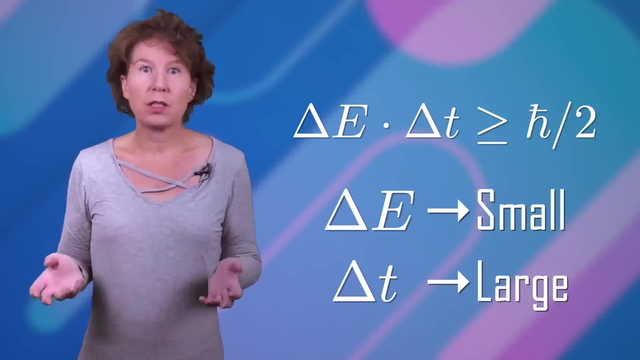 But what's the probability of it dropping down in a certain amount of time? And why is that? It's because you know something about the energy of the electron. It's sitting on this metastable level. Consequently, you can't know exactly how long it stays there. Such 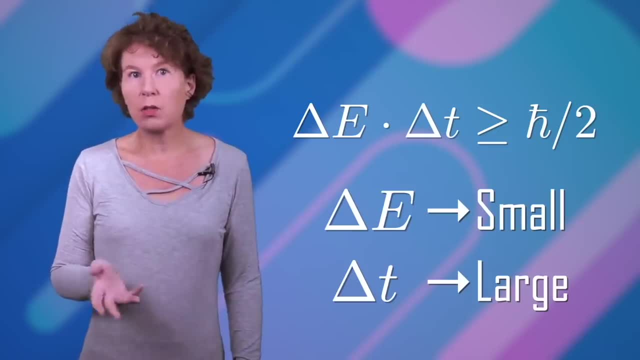 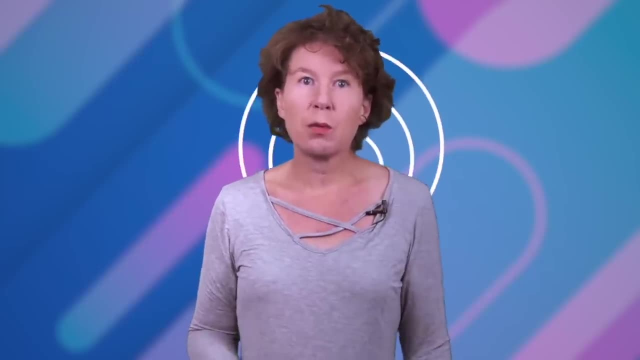 is life, you can't have it all. This is basically also how nuclear decay works, by the way. Finally, the uncertainty principle has its origin in the properties of waves. It comes about because, in quantum mechanics, particles can act like waves. 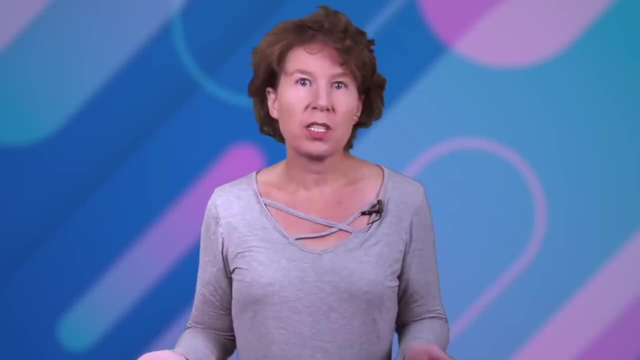 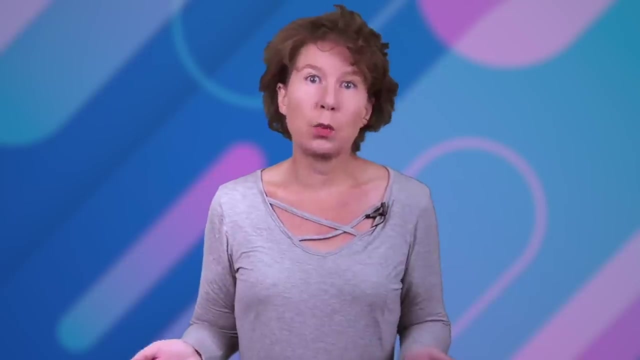 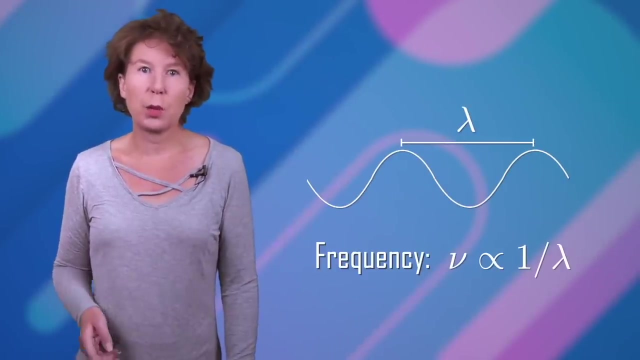 What's a wave? A wave is something that changes periodically in space and time. There could be water waves, electromagnetic waves, sound waves or even a Mexican wave when a sports game gets boring. Waves have a wavelength and a frequency that's inversely proportional to the wavelength. 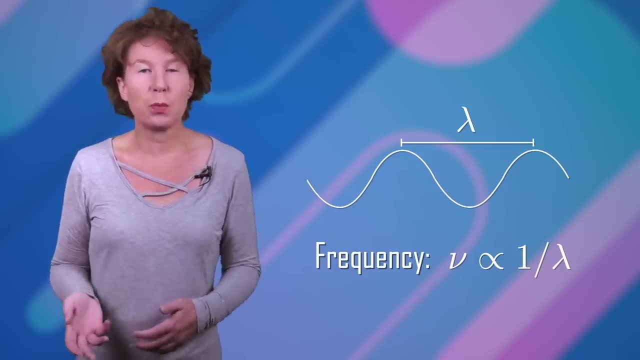 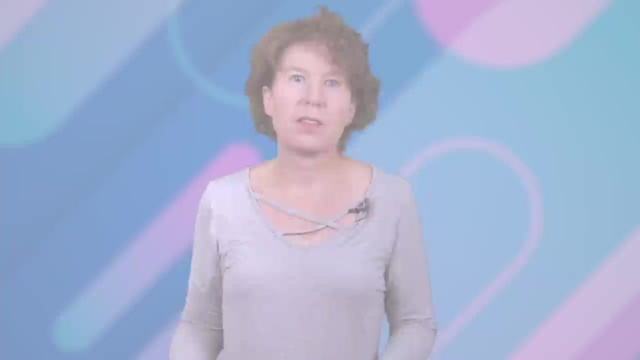 The frequency tells you how much change there is in a certain period of time. If you have a perfectly regular sound wave, then it would sound like a beep at one particular frequency. But most sound signals aren't that simple. For example, here's me singing an A. 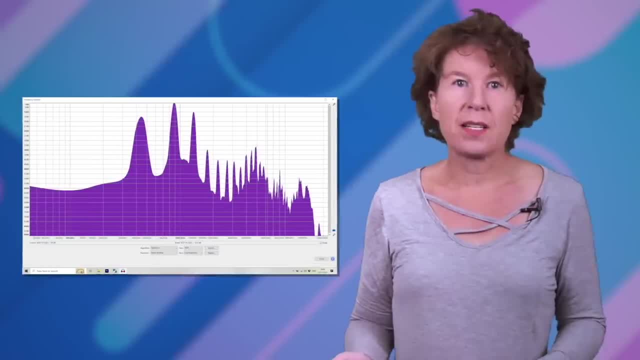 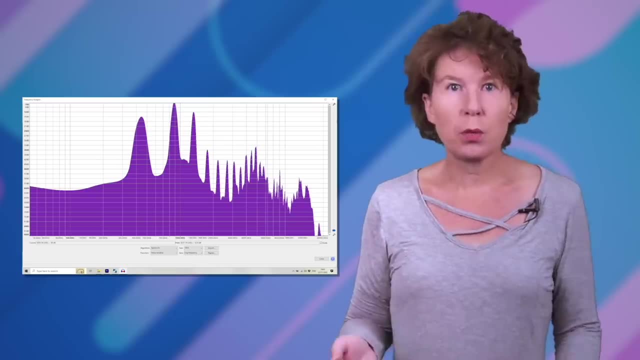 This isn't just one frequency. You can take this sound apart and you'll find that, for one thing, I'm not a computer chip, so I don't exactly hit the A, But also the way the human voice box works. it has a lot of higher harmonics. This breakdown of sound. 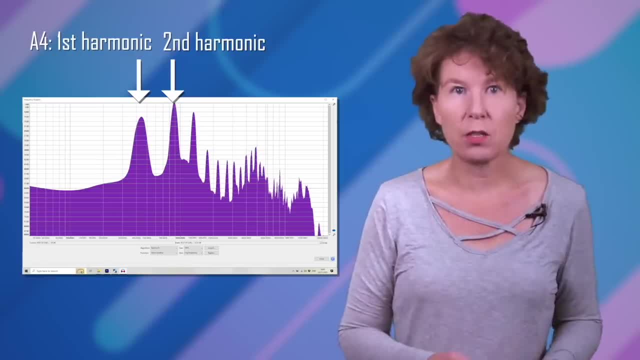 into all the frequencies it contains is very simple. I mean, you've got a lot of frequencies that you can't find anywhere else, so you can't exactly hit the A, But if you're means is called a spectrum. This doesn't only work for sound, but for every distribution of anything really. 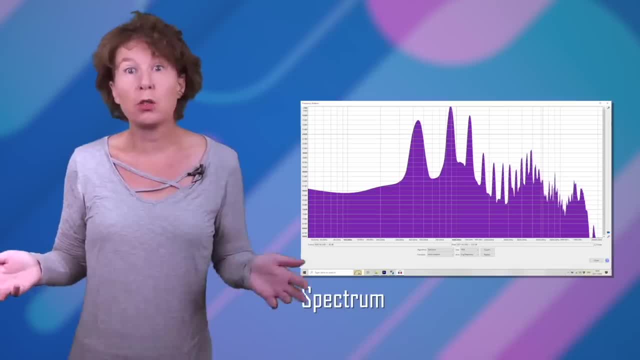 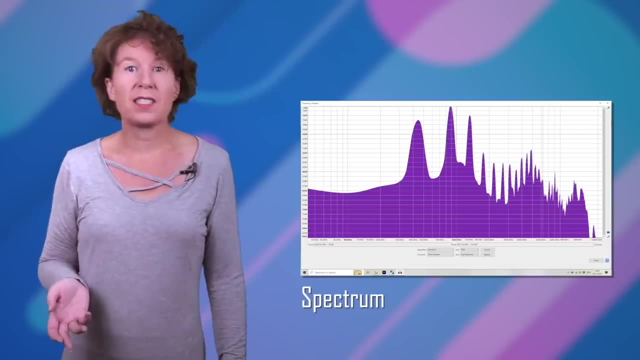 You can calculate a spectrum of the distribution of people in a room if you want to, and I'm sure somewhere there are physicists doing just that. But a more relevant example for us is light. If you have light of one particular wavelength, then that'd be one particular color, and 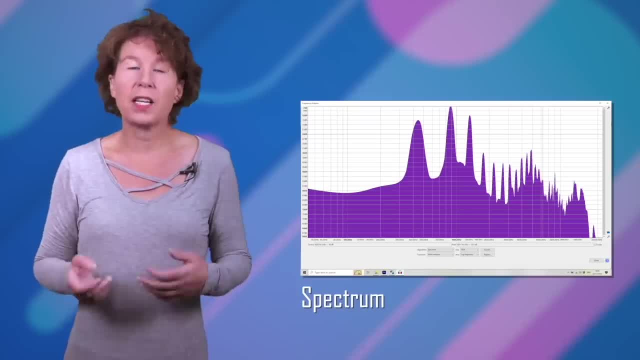 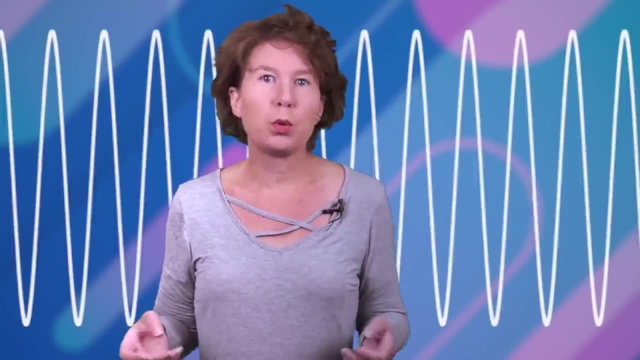 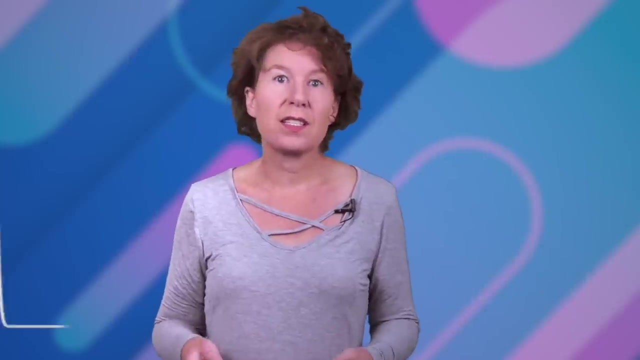 the spectrum of this light would have one single peak at one particular frequency. Technically, for the spectrum to be exactly one frequency, the light wave would have to keep on waving forever. We never deal with that in reality. In reality, the light we deal with is bunched. 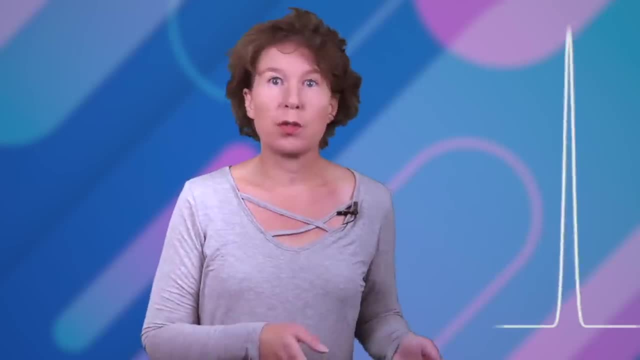 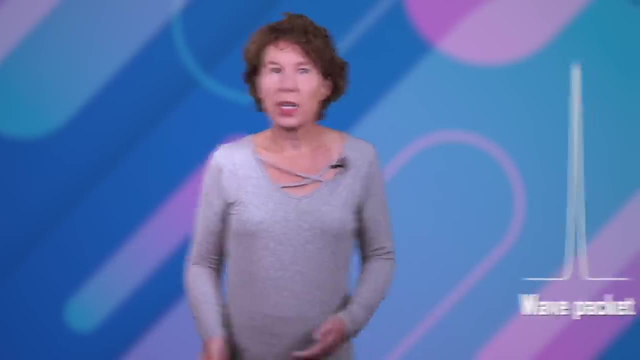 It passes by within a certain window of time. First it wasn't there, then it was there, now it isn't there again, like money on my bank account. Physicists call this a wave package. How do you pack waves, Especially without getting wet? 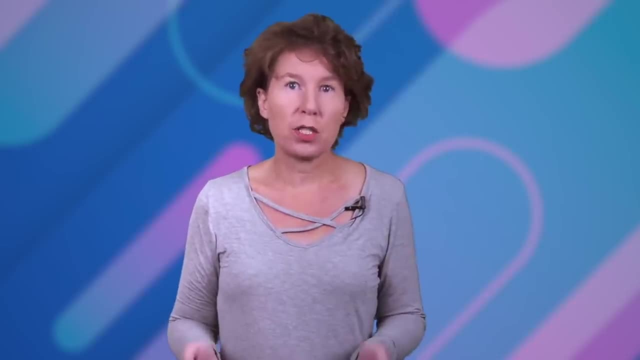 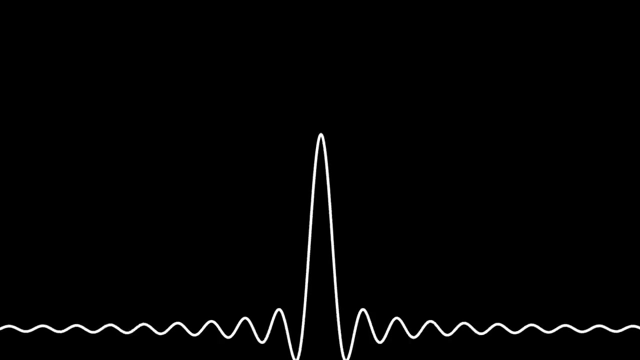 The curious thing about waves is that they can interfere both constructively and destructively. If they interfere constructively, they add up. If they interfere destructively, they can cancel each other out. If you overlay many of them in just the right way, you can do this so that, outside of some 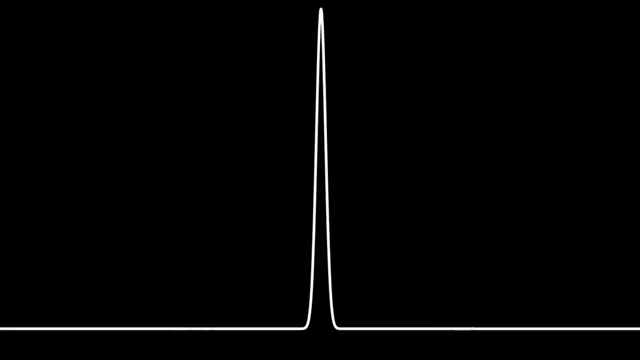 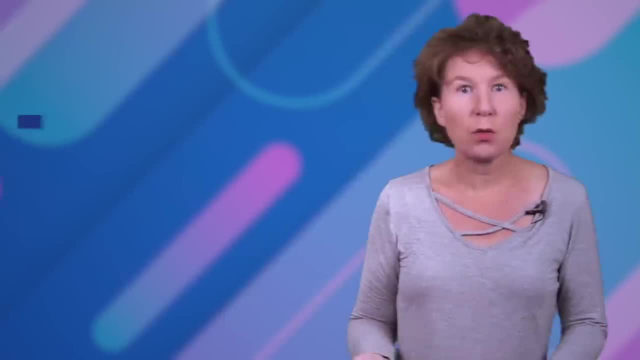 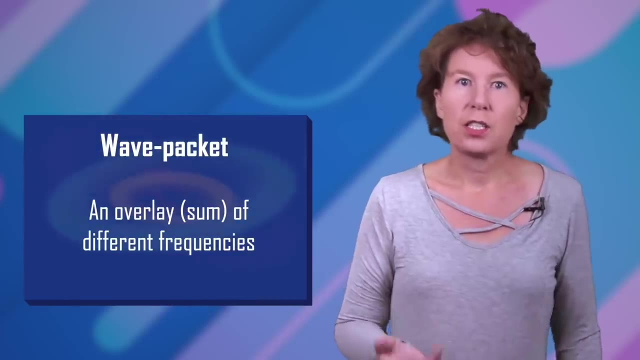 region of space and time. the interference is almost completely destructive and you are left with a constructive interference. A wave packet is an overlay of different wavelengths and therefore an overlay of different frequencies with the correct offset. Such an overlay, by the way, is called a superposition. 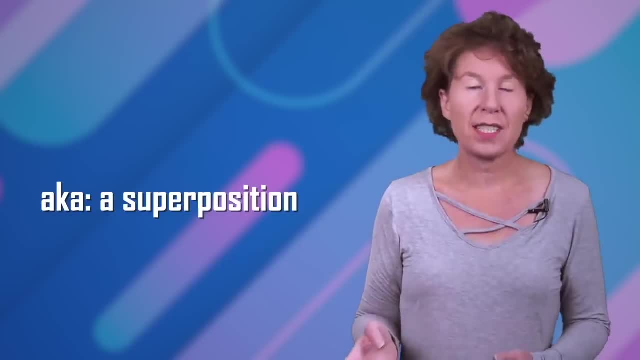 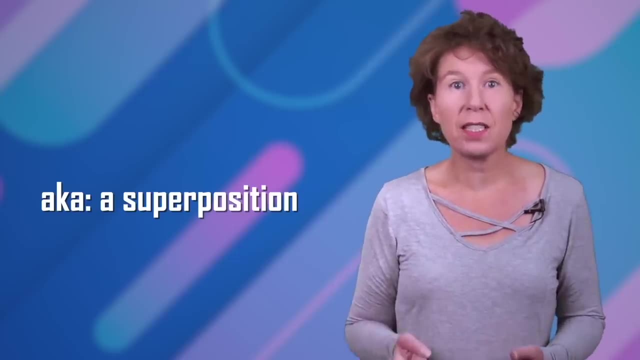 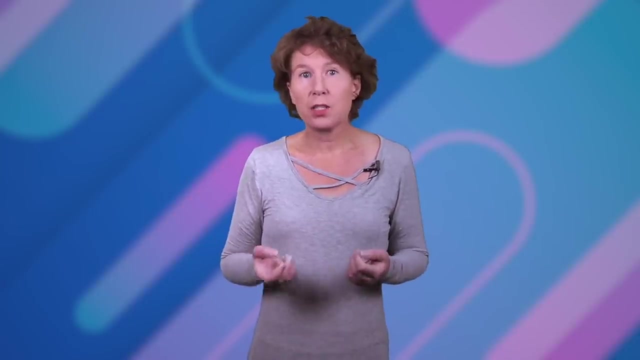 Sounds familiar. Yes, we do use superpositions in quantum mechanics, And this is where the word comes from. It comes from adding different wavelengths together. You superpose them. Okay. now here's the thing. Okay, So we have two ways to describe the same wave packet. 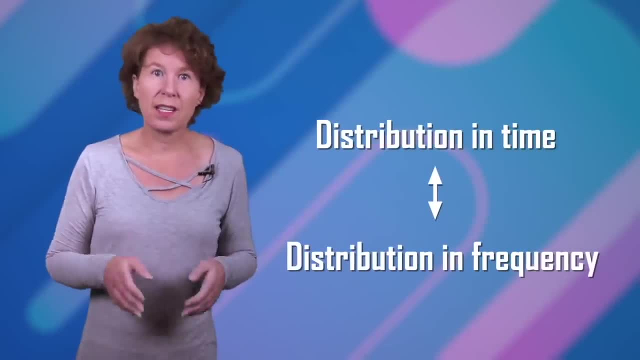 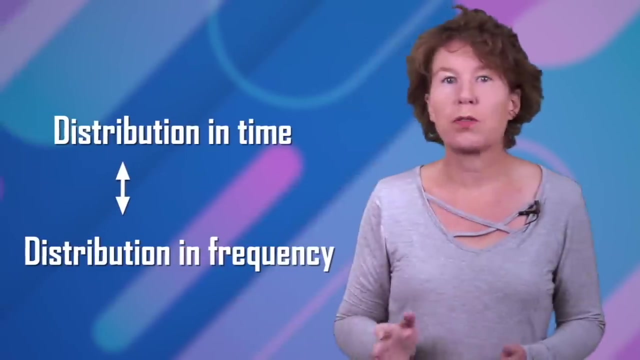 You can either say it's this distribution in time, wasn't there, was there, isn't there again, or you can say it's this distribution of frequencies with these offsets. They both describe the same thing, the same wave packet. There is a mathematical procedure to calculate one from the other. 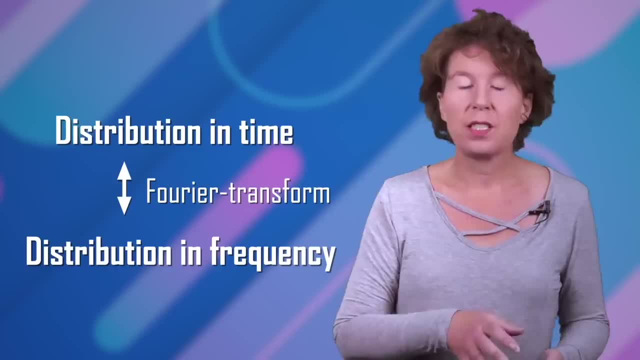 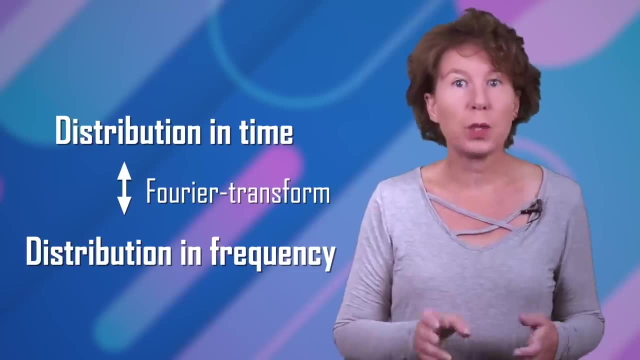 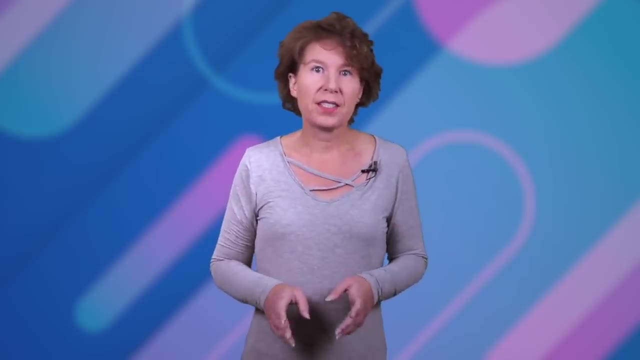 It's called a Fourier transformation. Put in a distribution in time, the Fourier transformation will give you the spectrum. put in the spectrum, the Fourier transformation will give you the distribution in time. Here's the kicker. If the one distribution is sharply peaked, say you have a flash of light. that's just. 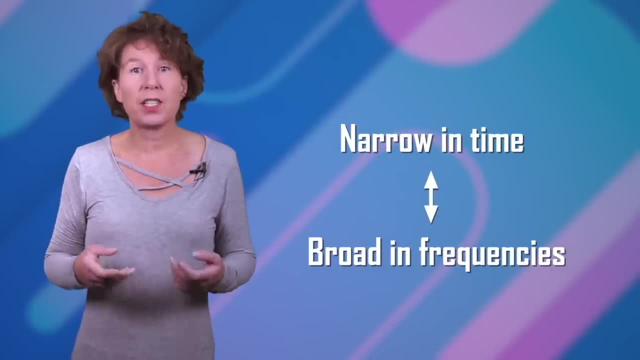 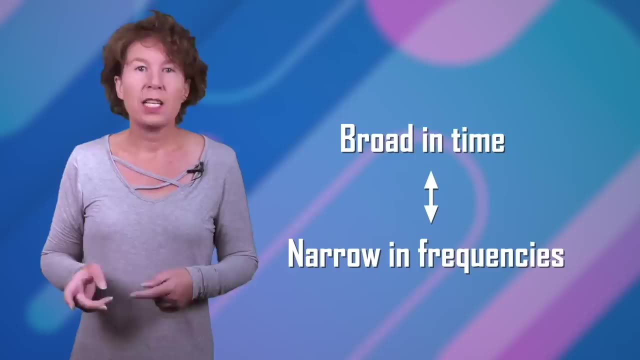 a brief moment in time, then that means that it must contain a lot of different frequencies. The spectrum is very spread out, And the opposite is also true. If you have something with a very narrow frequency, then it must be spread out in space. 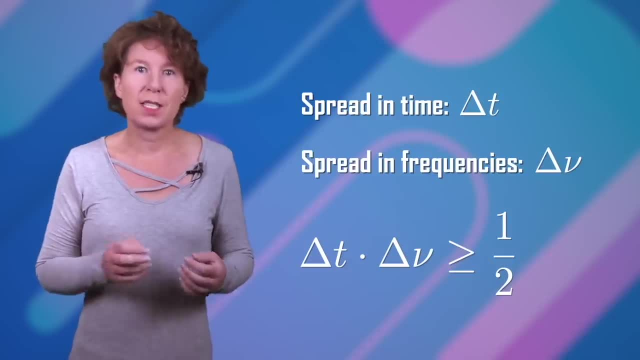 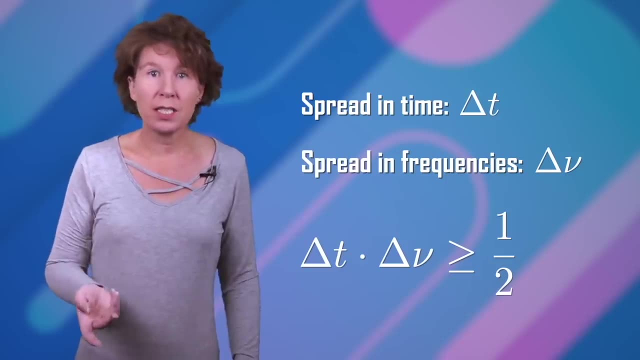 Now you can ask what's the relation between the spread in these two distributions, the one in time and the one in frequency? And, would you know it, they're related to each other by an inequality that looks pretty much like the uncertainty principle. 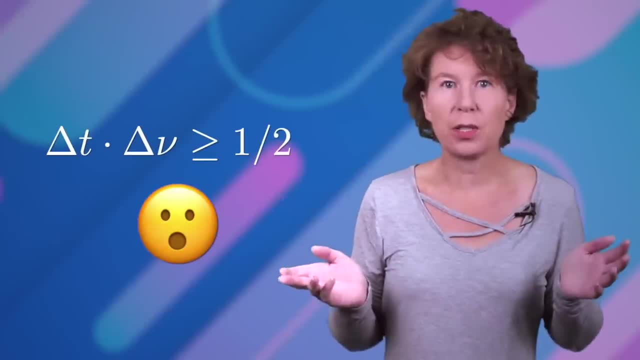 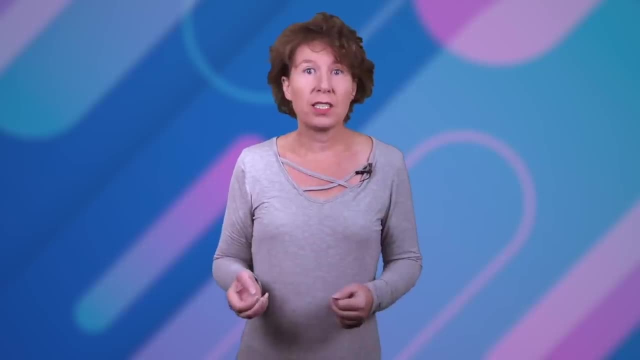 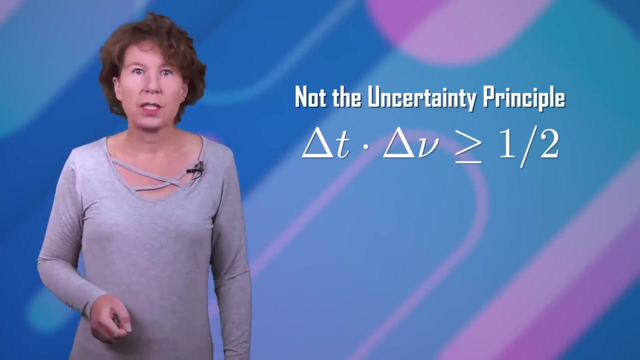 Whoa, But wait, This had nothing to do with quantum mechanics. We were just talking about spectral analysis. So what is going on? What's going on? is that why this looks like the uncertainty principle And why it's not? This is a property of waves. 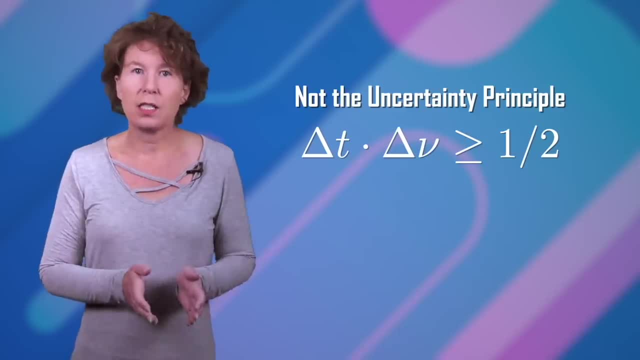 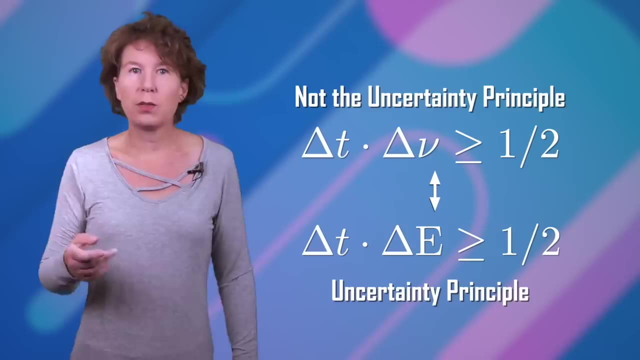 It relates a spread in time with a spread in frequency. To get Heisenberg's uncertainty principle, you further have to identify a frequency with an energy, Or, if you do it in space, you have to identify the wave vector with the momentum. 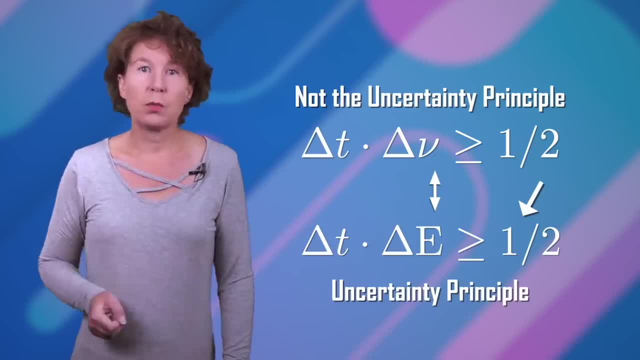 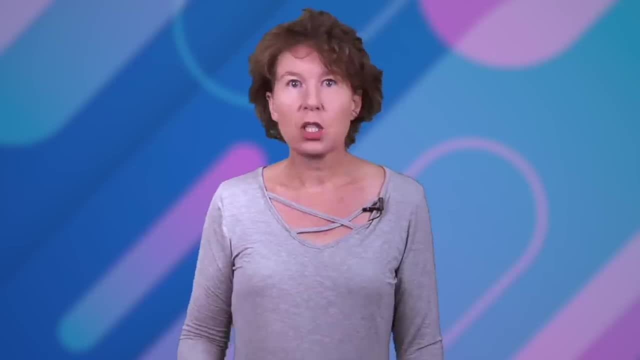 And this is where the H-bar gets in. We learned this from no other than Albert Einstein. Yes, that guy again, He pops up more than toast in a student house. He's a genius. It's actually what he won the Nobel Prize for. 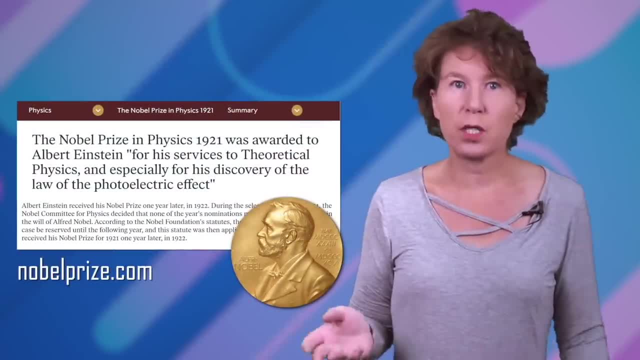 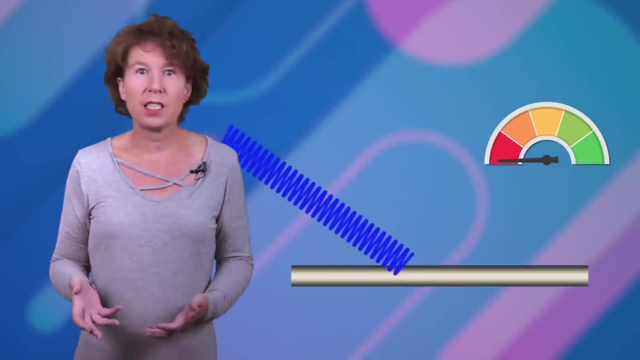 No, seriously, Albert Einstein didn't win the Nobel Prize for special or general relativity. He won it for putting H-bar in the right place, And the way he figured it out was from an observation called the photoelectric effect. If light shines on a metal plate, that can kick electrons out of the plate. 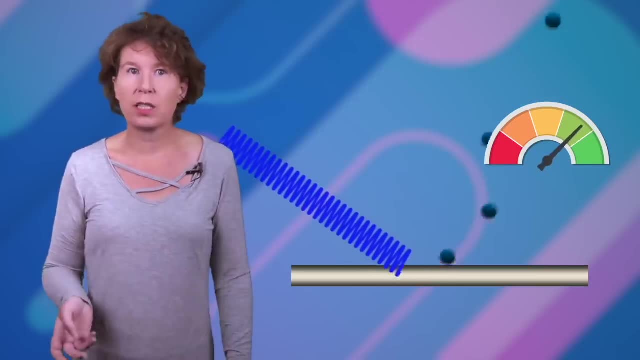 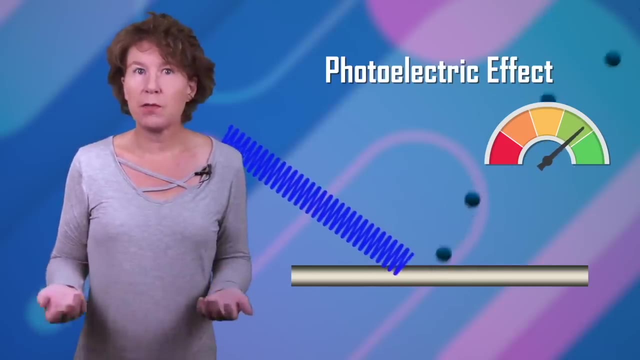 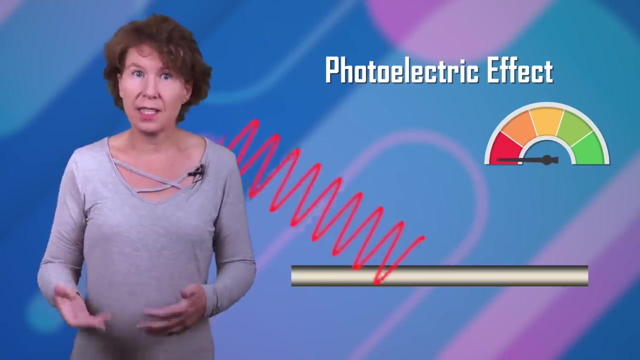 One can measure this because it creates a current, so it's electric. This is why it's called the photoelectric effect. But for this to work, the frequency of the light must be above a certain threshold. If the frequency stays below the threshold but you increase the brightness of the light, 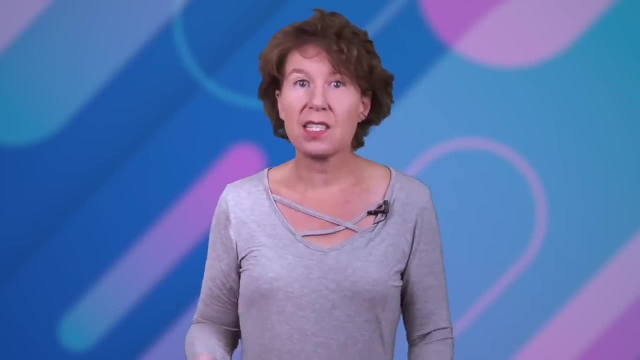 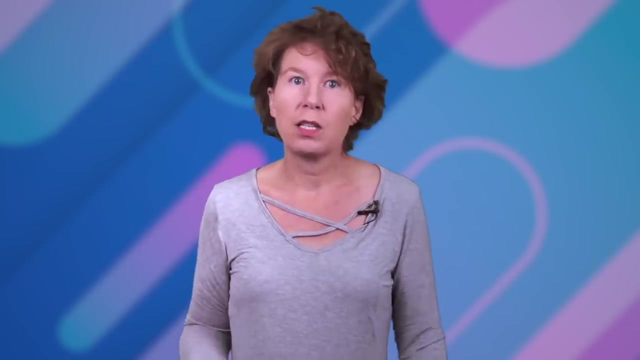 nothing happens. This was very confusing to scientists in the 19th century. They could understand that it takes energy above a certain threshold to kick out an electron, But if you think that light is a wave, then it's the brightness that measures this energy. 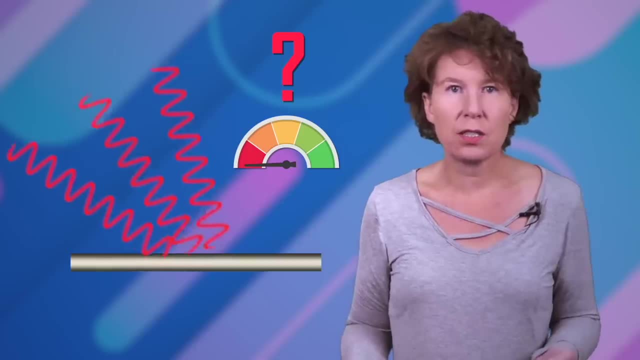 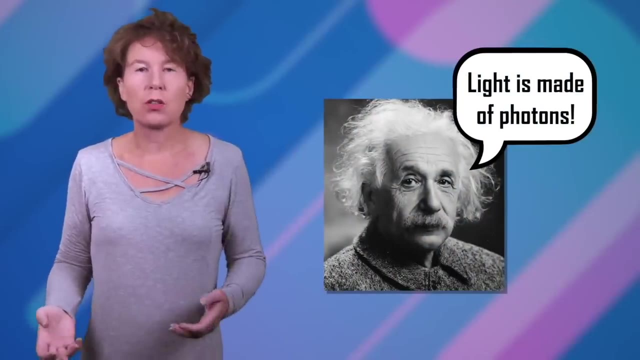 So why we're turning up the brightness, Not kick out electrons? Along came Einstein and he said that's because light is made of chunks of energy. We now call those chunks photons. To kick out an electron, the energy of the photon has to be above a threshold, not the 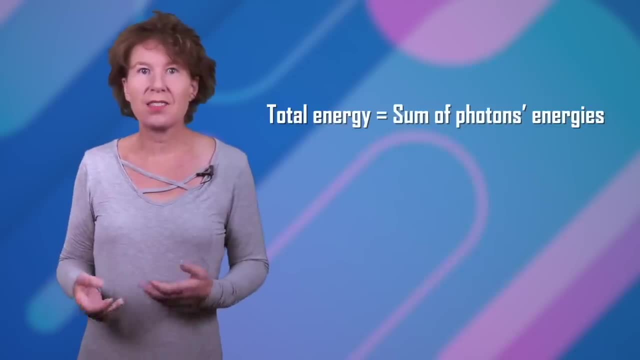 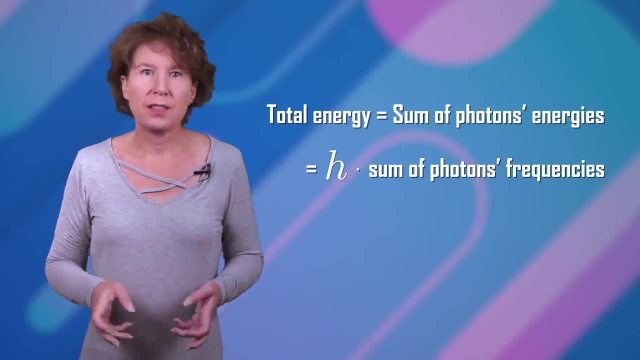 total energy of the light. The total energy of the light is the sum of the energy of all those photons, But the energy in each photon is proportional to the frequency. Therefore, if you want to know the total energy of the light, you have to know the total energy. 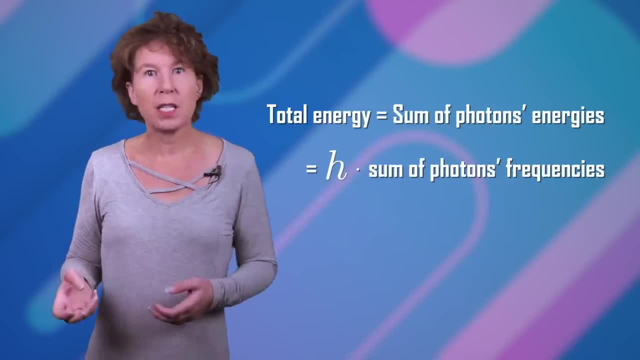 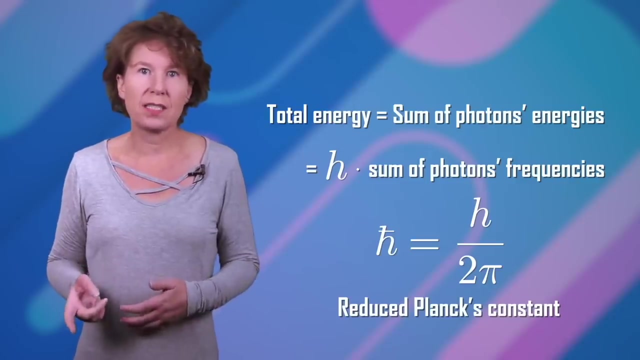 of the light. You take the number of photons and multiply it with their frequency, and now you need a constant to convert the frequency into an energy. That constant is Planck's constant, h And the h with the bar, that's called the reduced Planck's constant and is h divided. 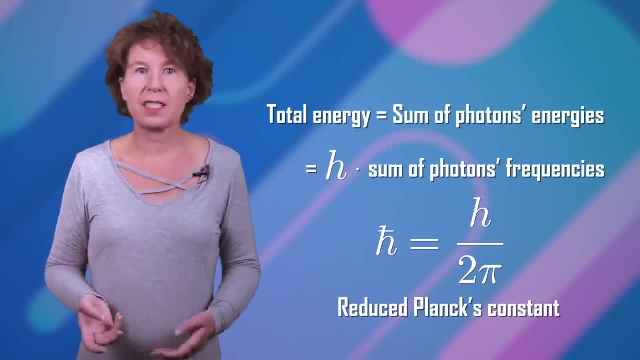 by two times pi. It's more commonly used in quantum mechanics because, like my uncle, it makes a lot of pi's disappear, so it's more convenient. Why is it called Planck's constant and not Einstein? Huh, good question, but I'll leave this for another video. 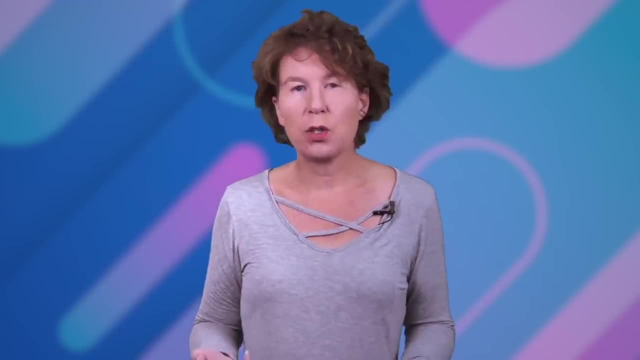 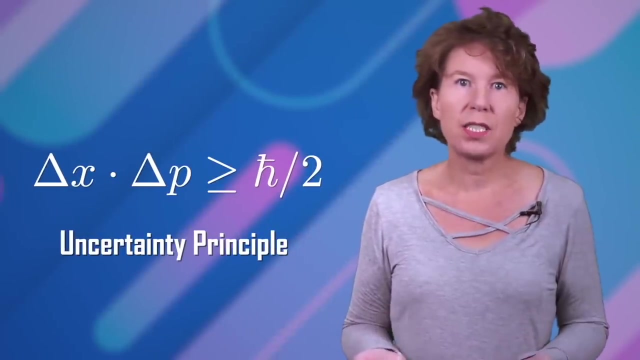 Let's instead step back here and ask what all this means. now We've seen that what's seemingly so weird about the uncertainty principle- that there are two quantities that you can't measure precisely at the same time- has really nothing to do with quantum mechanics. 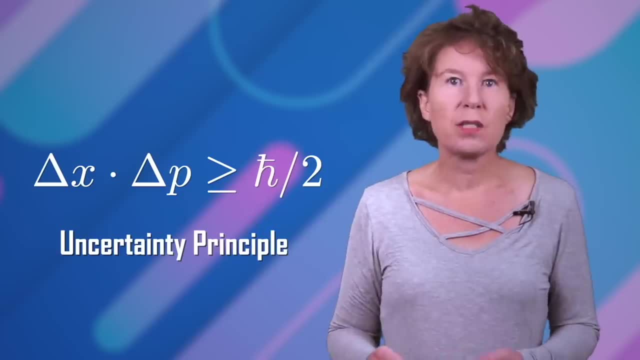 It's just a property of waves. What quantum mechanics does for you is to make this a property of particles, And that's why we call it the quantum mechanics. It's just a property of waves. What quantum mechanics does for you is to make this a property of particles. 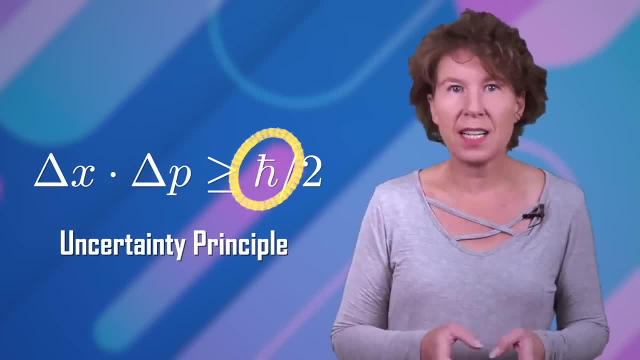 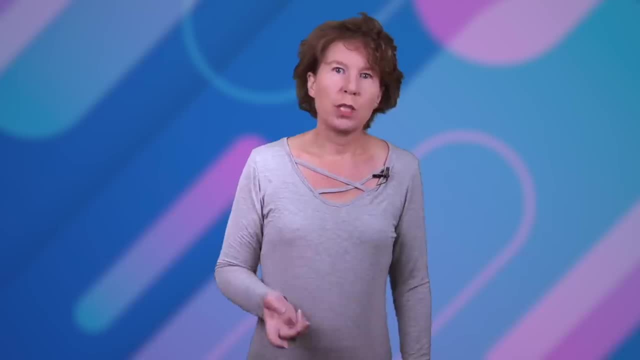 And for that to work you have to relate time with energy and space with momentum. If you're uncertain about any of this, then you're doing it right. We have also seen that the uncertainty principle doesn't mean you can't measure those quantities. 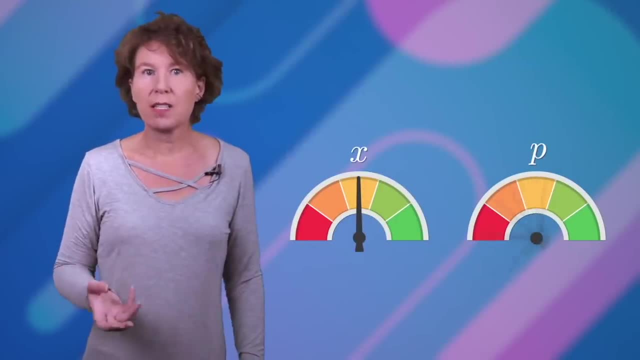 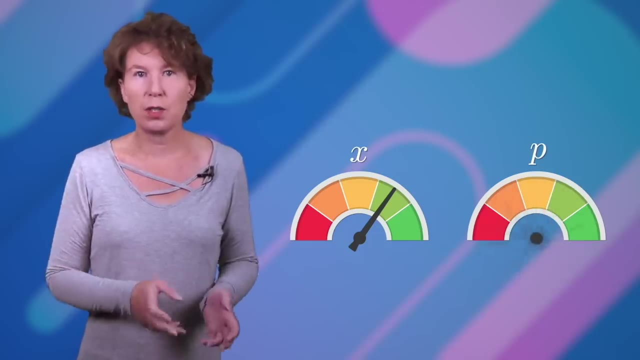 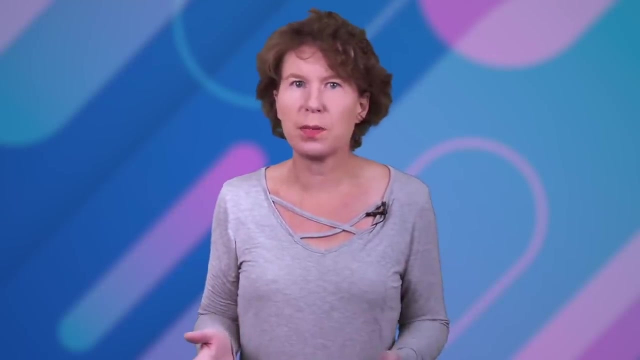 precisely in one round of an experiment. but that it means if you repeat the experiment you get a large statistical distribution for at least one of those quantities. But then couldn't it be The quantum particle actually had this property before it was measured? you just didn't. 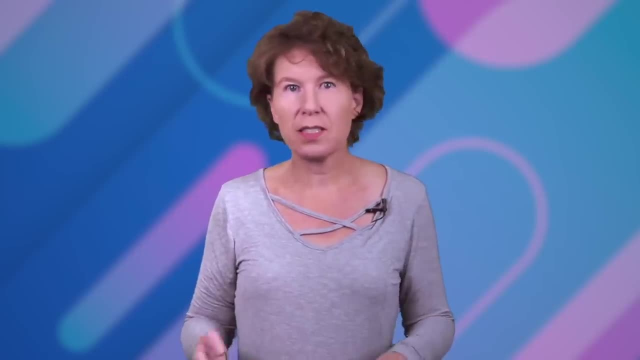 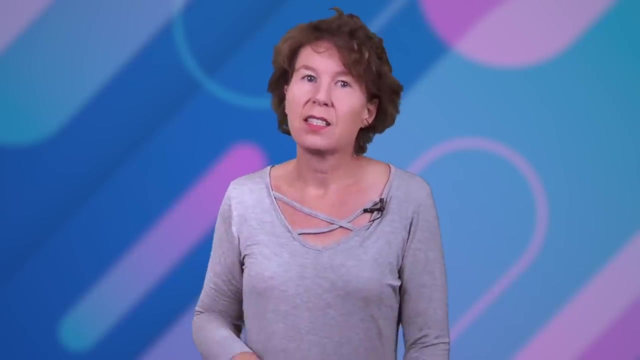 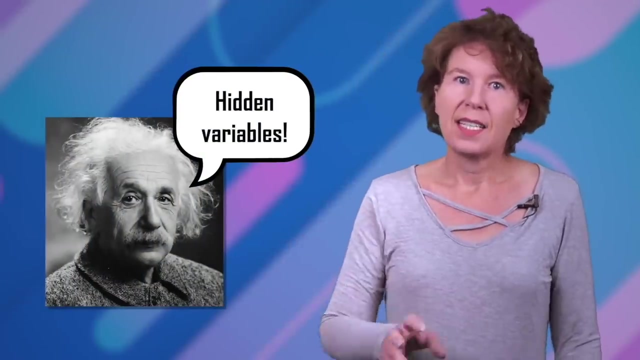 know what it was, Rather than doing this weird thing where it's in several states at the same time until you look at it and, poof, it decides on one. Yes, indeed, That's what is called a hidden variables model, And it's how Einstein thought quantum mechanics really works. 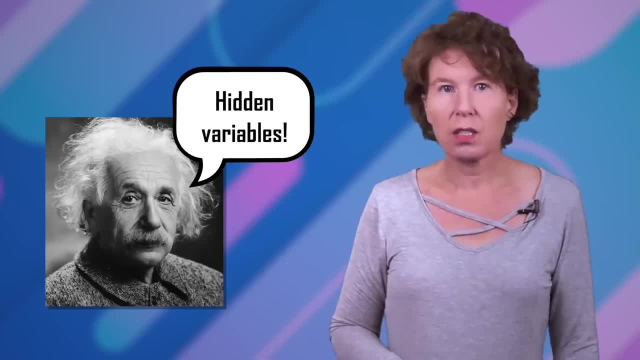 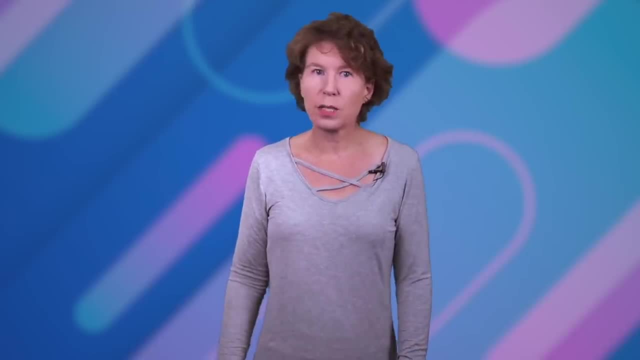 He didn't like spooky action at a distance And he was certain about his principles. I'm sure you've heard of quantum mechanics. I'm sure you've heard of it. I'm sure you've heard of it. It is great, especially if they're about such fun topics as quantum mechanics. 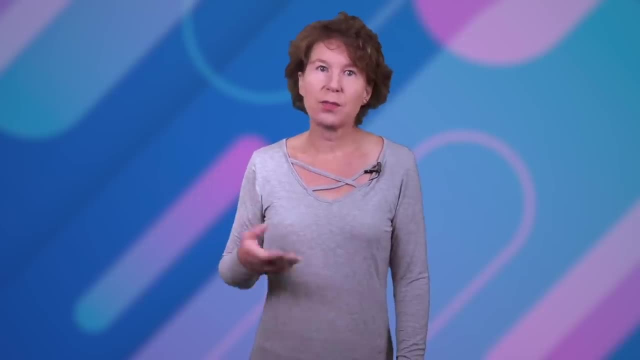 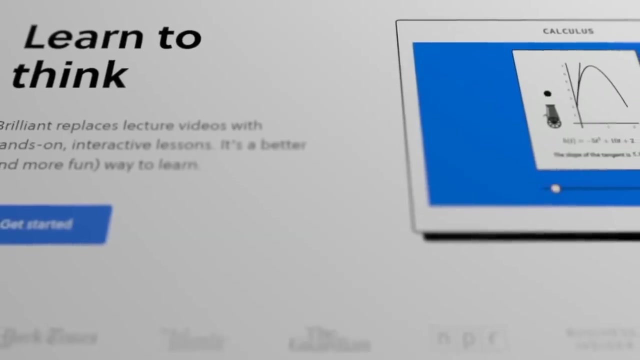 But if you want to really understand a topic then you have to actively engage with the material. A great place to do that is Brilliant, who have been sponsoring this video. On Brilliant you find courses on a large variety of subjects in science and mathematics. 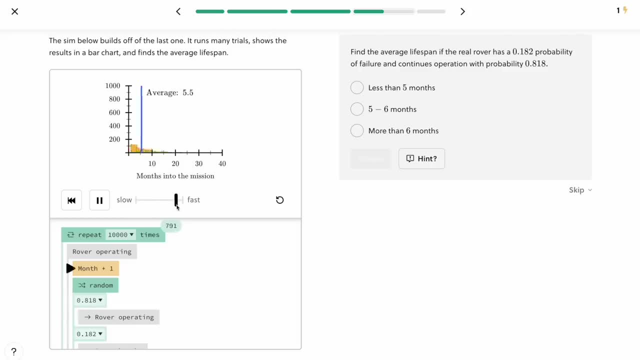 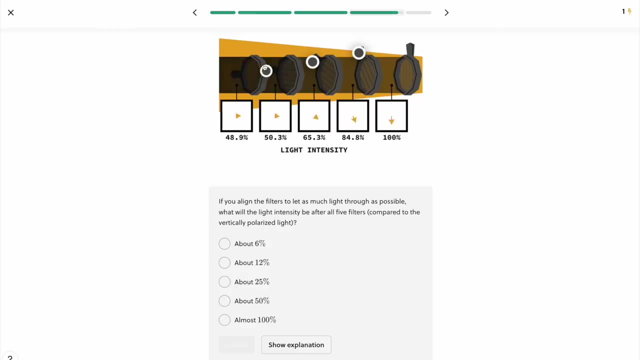 The great thing about their courses is that they are all interactive, with visualizations and follow-up questions, so you can check your understanding right away. This is why I like to look things up on Brilliant. it's fast, it's easy and it tells me. 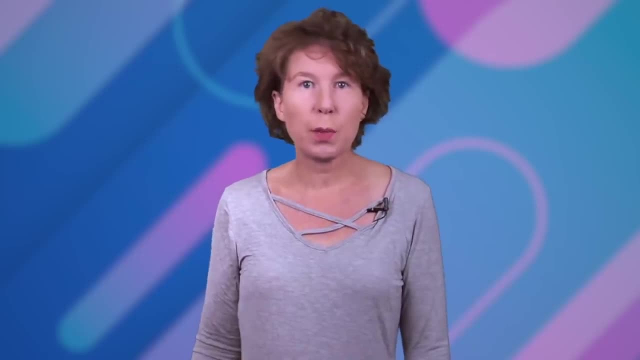 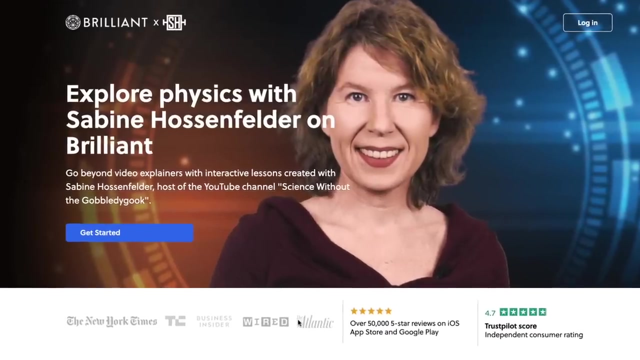 what I need to know, And they are constantly expanding their content To understand better what I talked about in this video. check out, for example, my course about quantum mechanics. It gives you an introduction to interference, superpositions and entanglement and, of course, 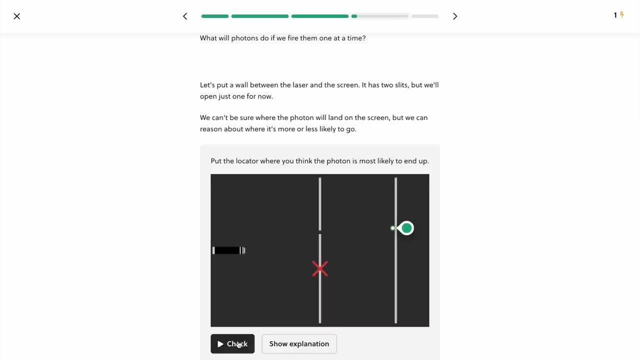 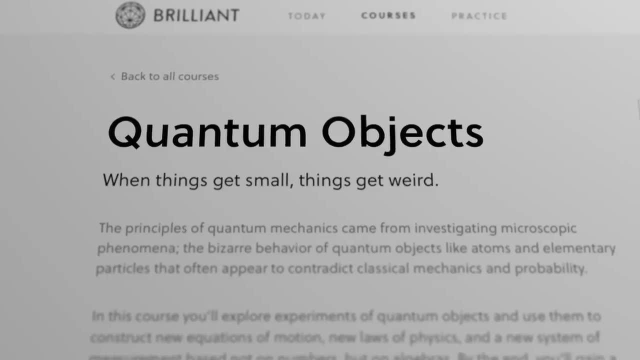 the uncertainty principle. It begins from the very basics, So you don't need to bring any background to it. I hope you enjoyed this video. I hope you enjoyed it And after that you can continue, maybe with their course on quantum objects or quantum.